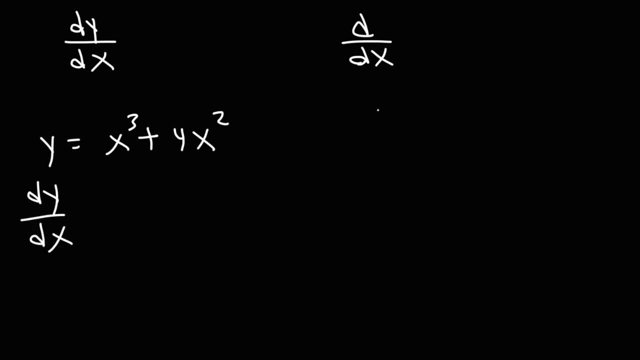 What does it mean when you see dy dx in a problem like this? And sometimes you'll see this d of dx and then x cubed plus 4x squared. So what's the difference? Well, here's the way I like to think about it. 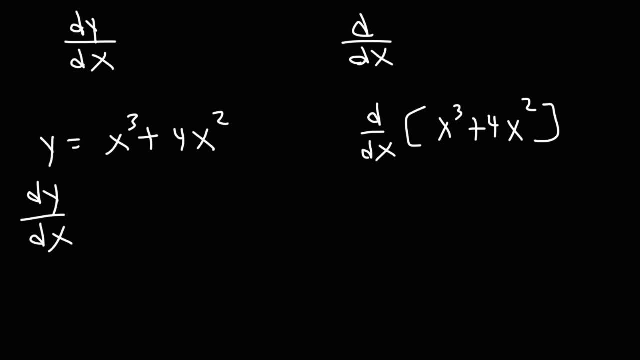 dy dx kind of tell me what it is. d over dx tells me what to do. d over dx expresses a command. It's basically saying: hey, find the derivative of whatever's inside of here with respect to x. dy over dx tells you: hey. 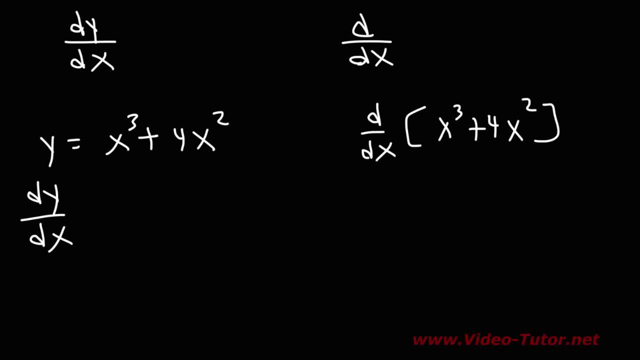 this is the derivative of whatever's inside of here. with respect to x. This is the derivative of whatever's inside of here. with respect to x. This is the derivative of some function, in this case y. The derivative of y with respect to x is 3x squared plus 8x. 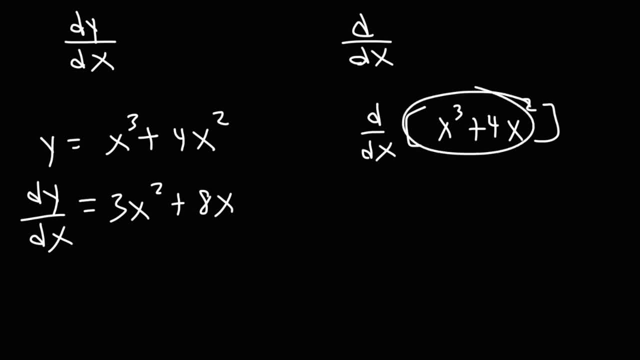 And in this case this expression tells us to differentiate this expression, which will be the same thing: 3x squared plus 8x. So hopefully that kind of helped you to see the difference between the two. So d over dx tells you. 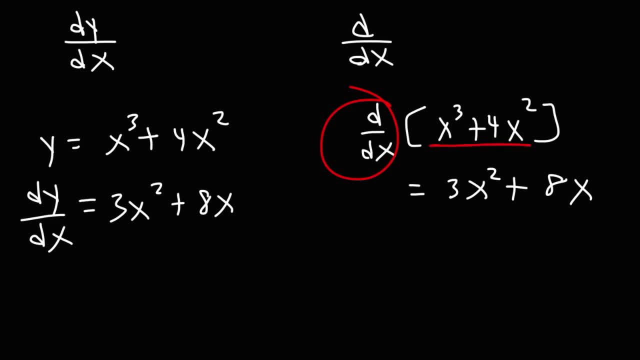 what to do. It tells you to differentiate the function inside the brackets with respect to x, dy, dx simply makes a statement. It tells you that the derivative of y with respect to x is equal to whatever you see here. Now let's see if we can put this together. 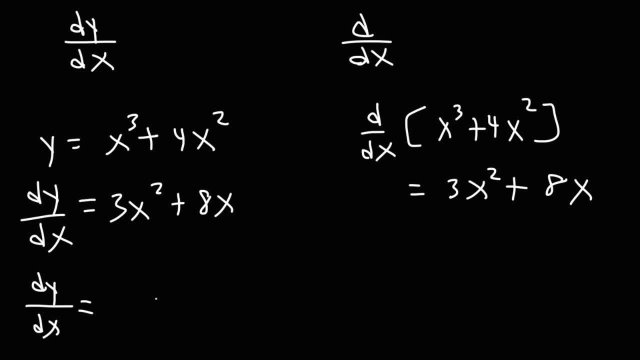 dy over dx is equivalent to saying: take the derivative of y with respect to x And we can put this together. And we can replace y with this expression: y is x cubed plus 4x squared. Using the power rule, this is going to give us 3x squared plus 8x. 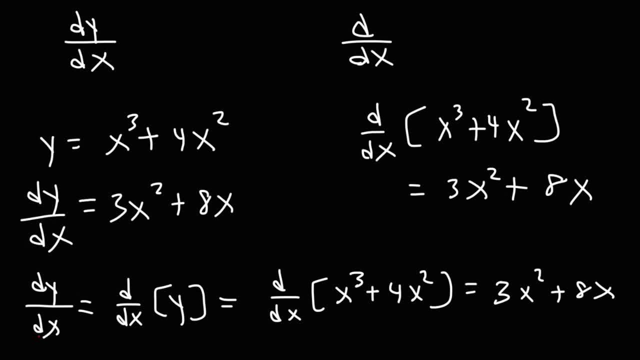 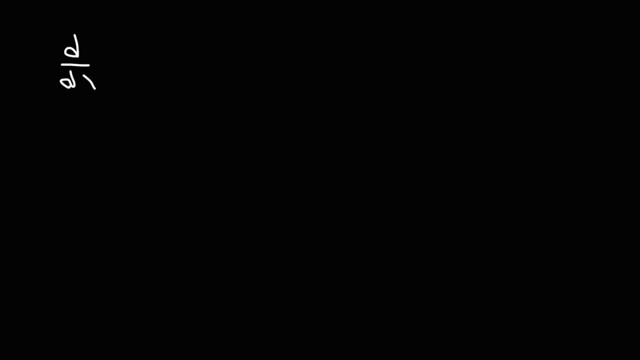 Which, as we can see, that's equal to dy over dx. So hopefully that connected everything together when you see these two things Now. now, if we want to find the derivative of x cubed with respect to x, we know it's 3x squared. 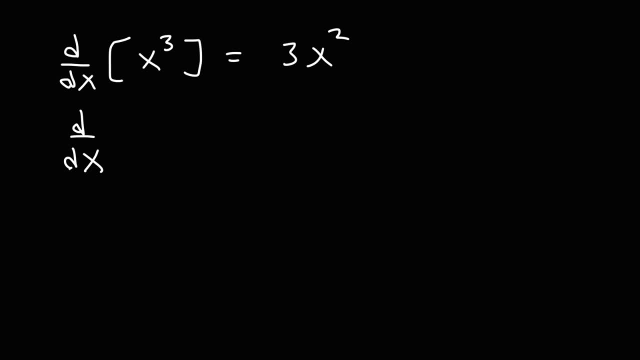 But what if we want to find the derivative of, let's say, y cubed with respect to x? What's the answer? Well, using the power rule, it's going to be 3y squared. But notice that these variables do not match. 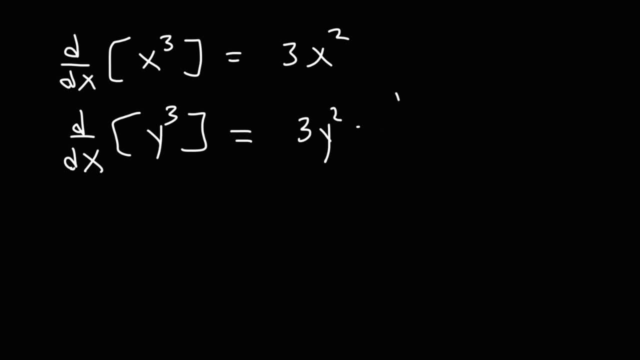 So we're going to have something else. It's going to be 3y squared times dy, So we're going to have 3y squared over dx. Typically, you'll see problems like this when dealing with something called Implicit Differentiation. 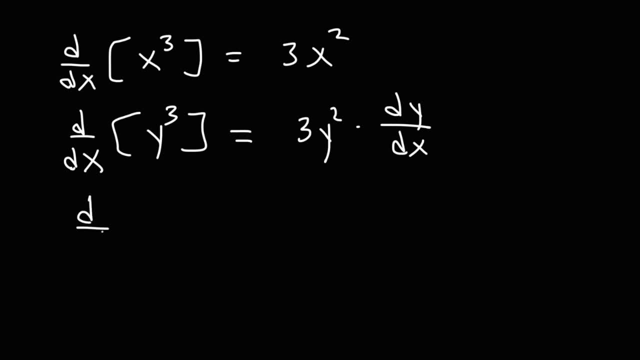 Now what if we want to differentiate, let's say, x to the fifth power with respect to some variable s? This would be 5x to the fourth times dx, ds. So that's the derivative of x with respect to s. Now, sometimes, when dealing with related rates problems, you'll see d over dt. 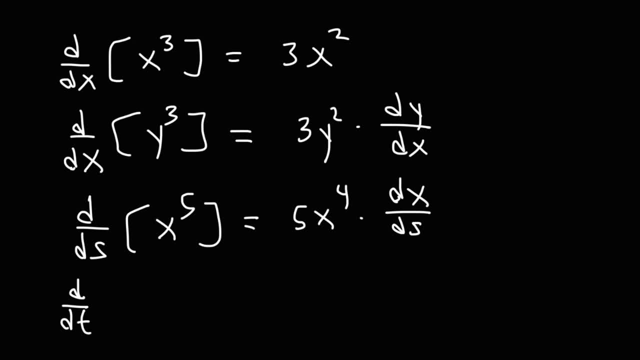 So you're differentiating with respect to time. So you could differentiate with respect to many things. You could differentiate with respect to x, with respect to some other variable, s or with respect to t. So let's say, if we want to differentiate x to the fourth power plus y cubed, with respect to time. 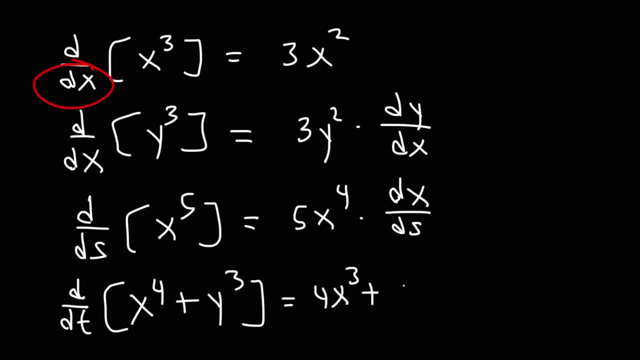 it's going to be 4x cubed Plus 3y squared. Actually, let's take that back. It's 4x cubed times dx dt And then plus 3y squared times dy dt. So dx dt is the derivative of x with respect to time. 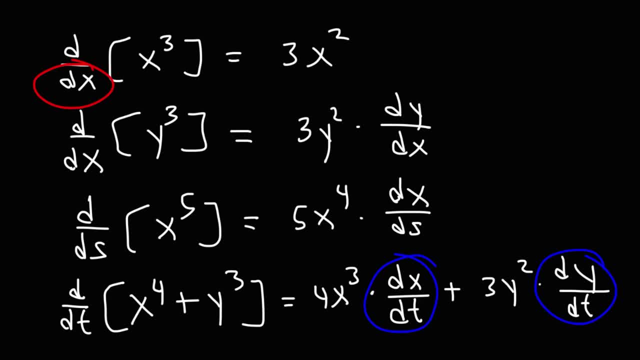 dy, dt is the derivative of y with respect to time, So I don't know if you've covered related rates yet, But you'll see that a lot We're dealing with that topic. Okay, time for a pop quiz. Let's see if you've been paying attention. 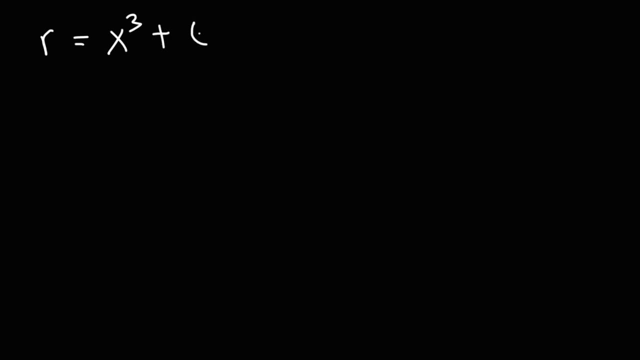 Let's say that r is a function of x and t And that r is equal to x cubed plus t to the fifth power. Go ahead and find dr over dy. Feel free to pause the video if you want to try this problem.